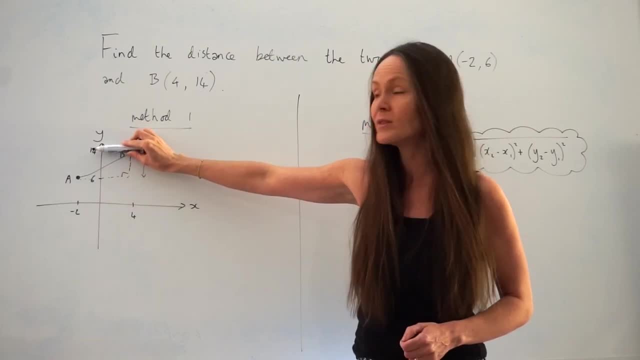 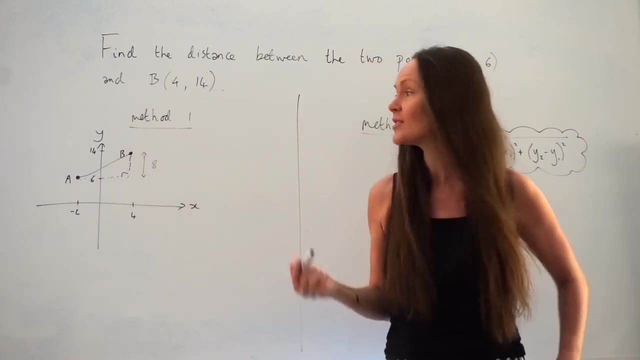 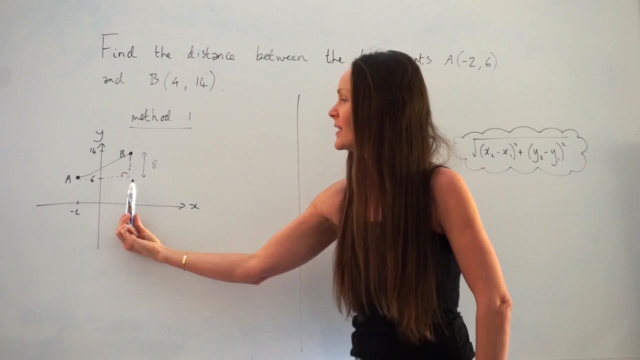 with positive 6 and point B is in line with 14 along the y-axis. So the difference between 6 and 14 is 8.. So that's the height of our triangle. Now, if we look at the base, you can see point A is in line with negative 2, point B is in line with 4.. So that is a base of. 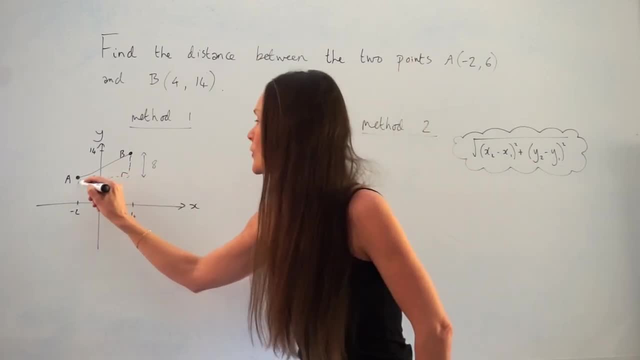 6.. The difference between minus 2 and 4 is 6.. So we've got the length of the base, we've got the height of the triangle. we've got the length of the base and we have the height. So from there you just do the square root. 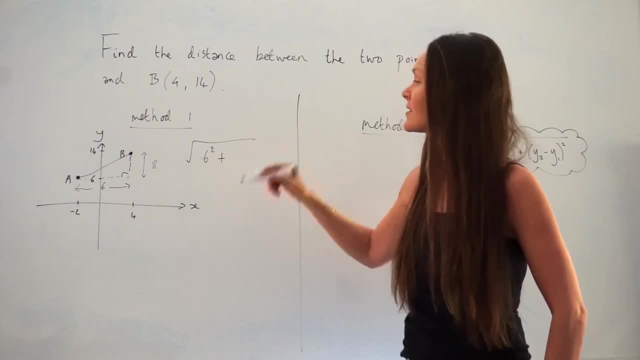 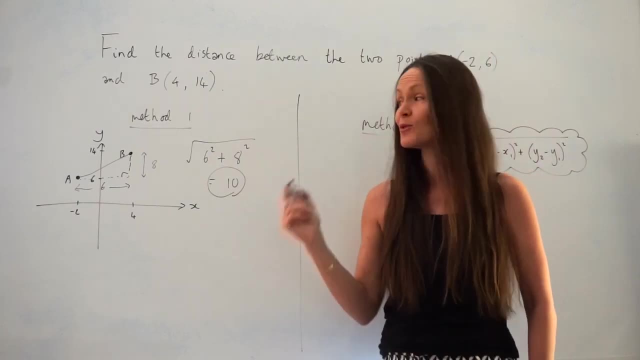 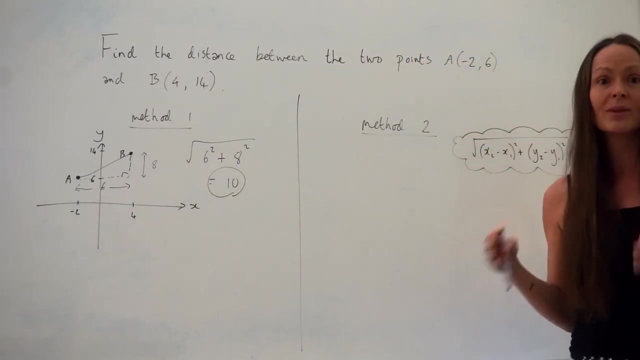 of the base squared, which is 6 squared, plus the height squared, which is 8 squared, and if you calculate that, you get 10.. So that is the distance between the two points, just using a sketch and Pythagoras' theorem. Now, method 2 is essentially the same. We're still. 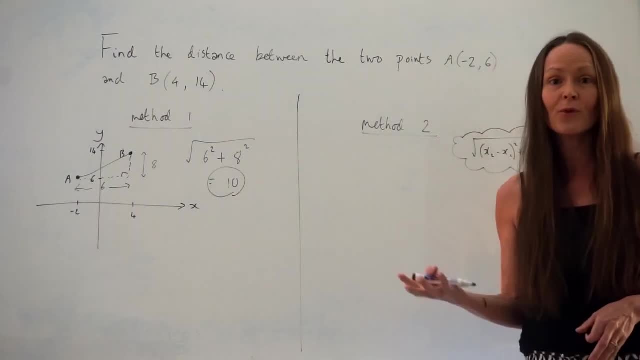 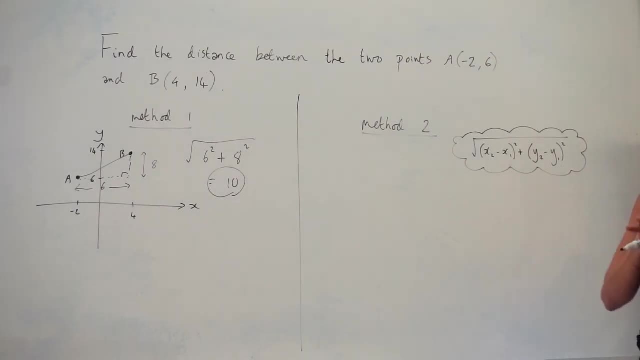 using Pythagoras' theorem, but without the sketch and using a formula, And sometimes this is the preferred method, Because they might give you this formula in the formula booklet, Or maybe you're just a pro at remembering formulae. So in this formula it says the square root of the difference. 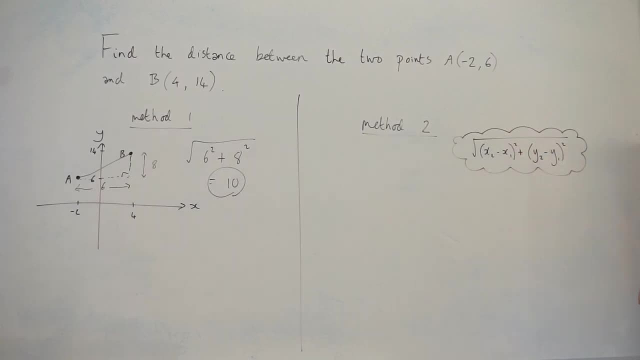 between the x values squared plus the difference between the y values squared. So let's just identify which point is going to be x1, y1 and which one is going to be x2, y2.. So I'm going to take point A and I'm going to label this x value x1, which means this one has to. 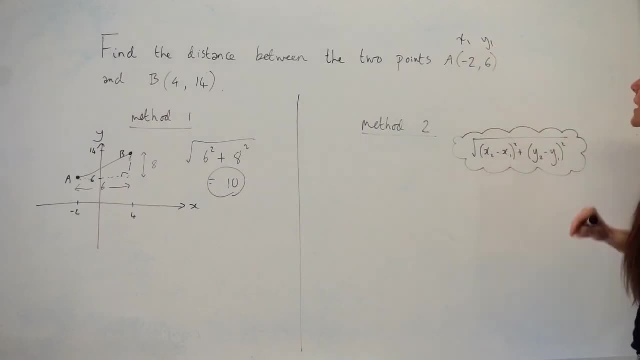 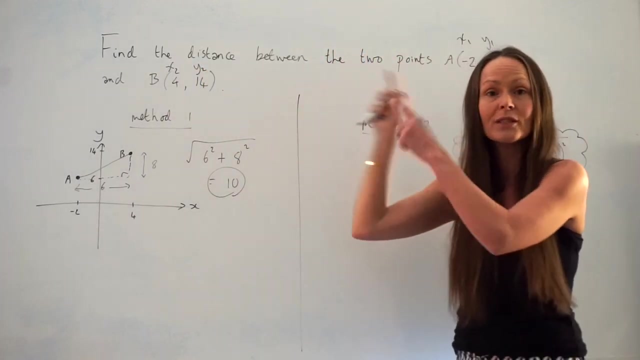 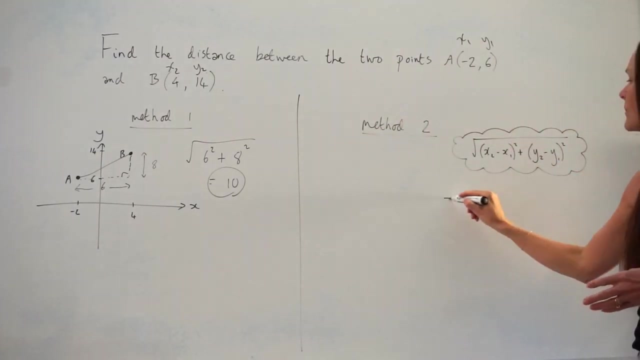 be y1.. So I've got the 1s for this point here, which means the other point has to be x2 and y2.. And it doesn't matter if you did those the other way around. Now all you're doing is substituting those numbers from the coordinates into the formula. So we're doing the square. 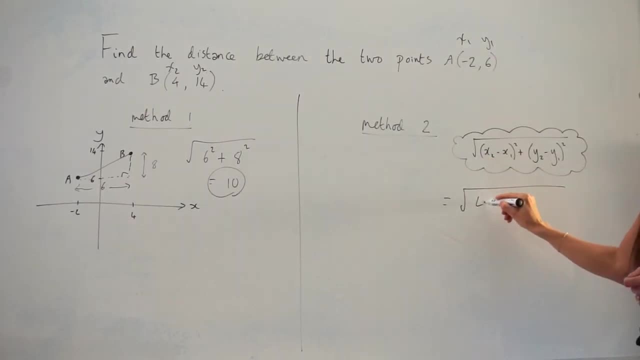 root of x2, which is 4.. Take away x1, which is negative, 2 all squared. Remember, you're always subtracting, So finding the difference between the x and the y values squared. So you're working out a difference between the x values, Just like we did there in our sketch. 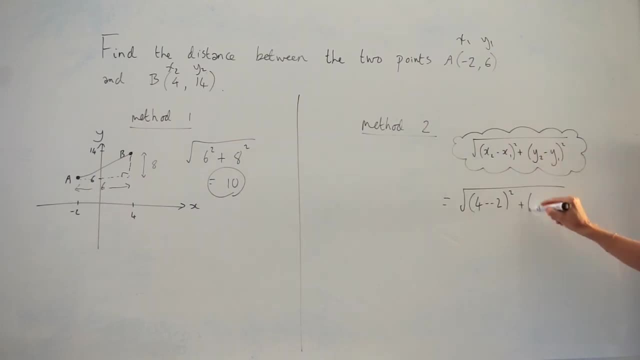 okay, Then you're adding- remember it's Pythagoras' theorem, so it's still adding in between. And then you're working out the difference between the y values, So y2 is 14 and y1 is 6.. Remember you're subtracting in this specific order. And then don't forget to square And. 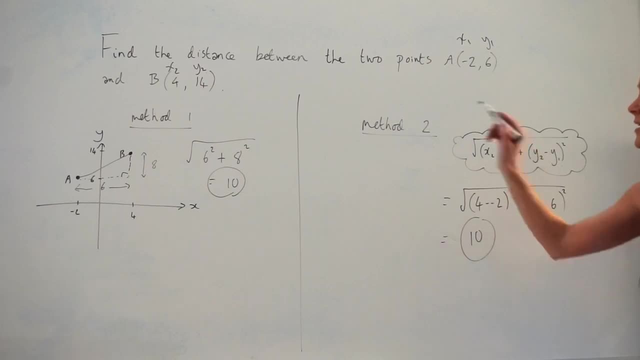 obviously, if you work that out, you're going to get the same answer as in Method 1, which is 10.. So in the next question it says Qkäist voix, Two times four rents. Väl Eating === Meantime. you have tres'. 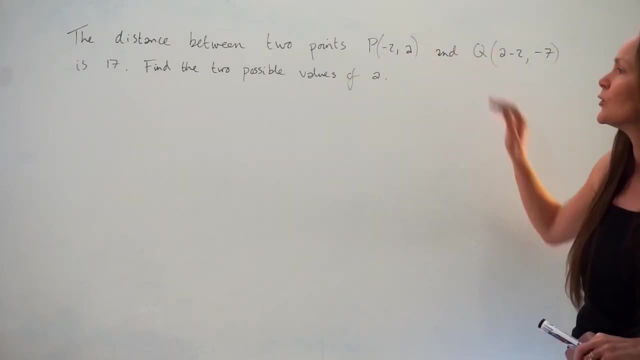 Four times a woman, except six. Quotation of four minutes. preference elevenths partiality, which is a patience number' the distance between the two points P and Q is 17.. So the coordinates of P are minus 2A and the coordinates of Q are A minus 2 minus 7.. In this question we have to find: 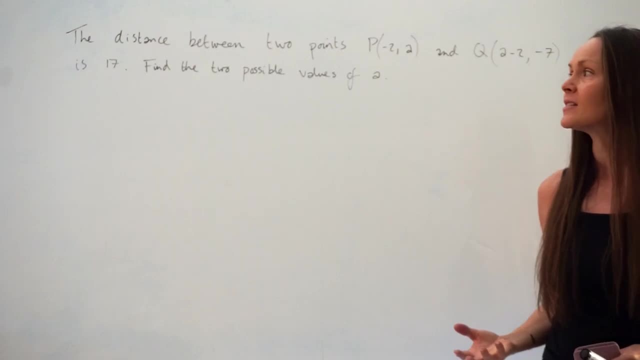 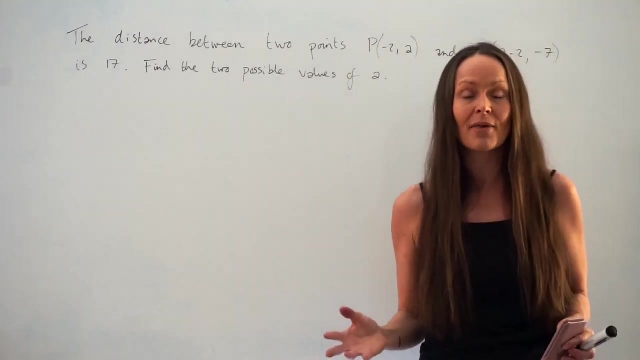 the two possible values of A. So they've given us the distance between the points, which is 17,. but we don't know the precise coordinates. So I would avoid using the sketch method on this question, as it might be a little bit confusing where you're going to plot the points. 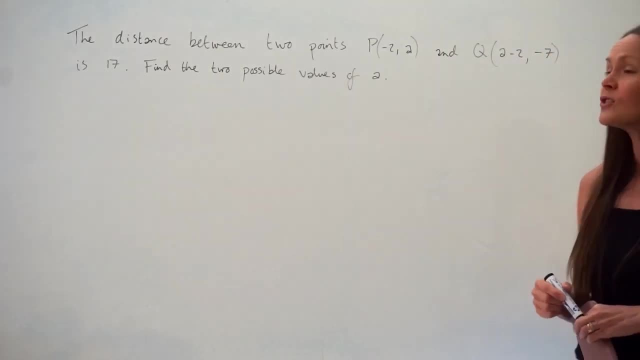 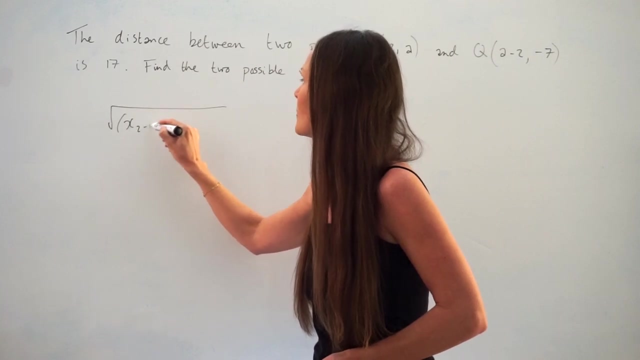 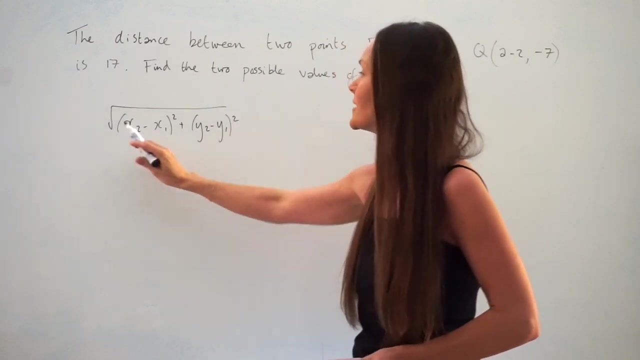 if you don't know the exact coordinates, So we're going to use method 2.. So I'm going to start by writing down the formula. So the square root of X2 minus X1 all squared, plus Y2 minus 1 all squared, So it's just the difference between the X value squared plus the difference. 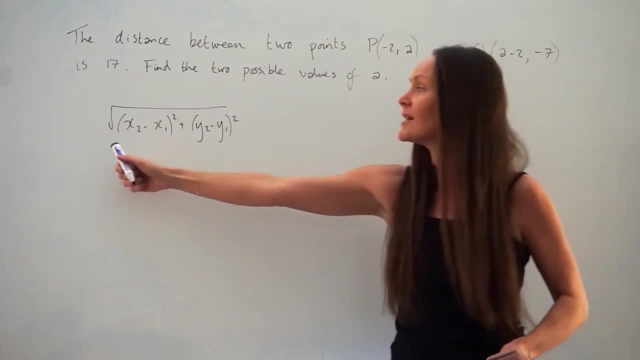 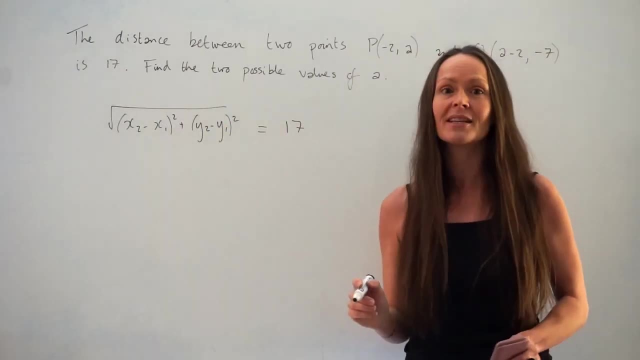 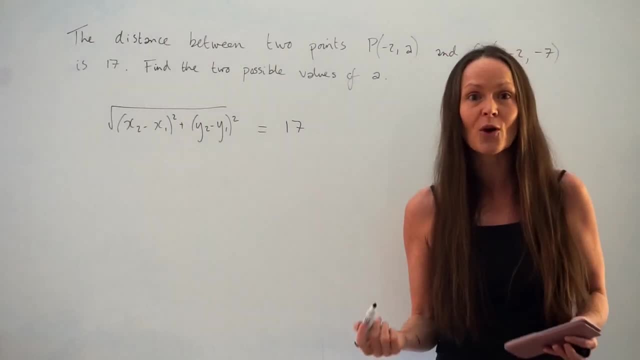 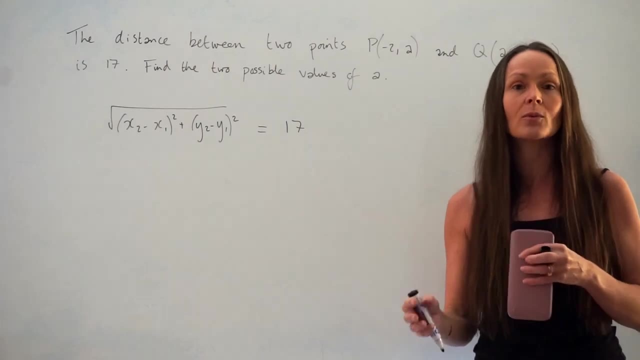 going to put this in the equation. So I'm forming an equation that hopefully later I can use to solve and find the two values of A. So to begin with I'm going to decide which coordinates are X1, Y1, and X2, Y2.. So let's say P is going to be X1, Y1, and 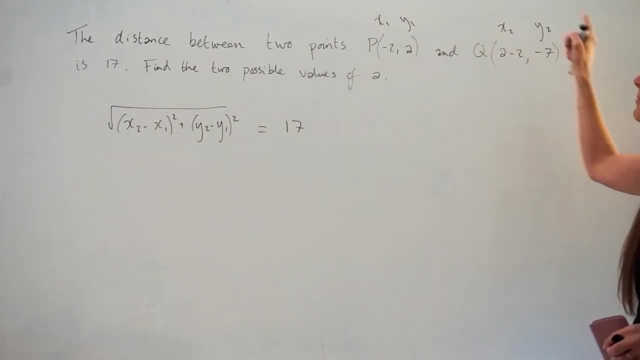 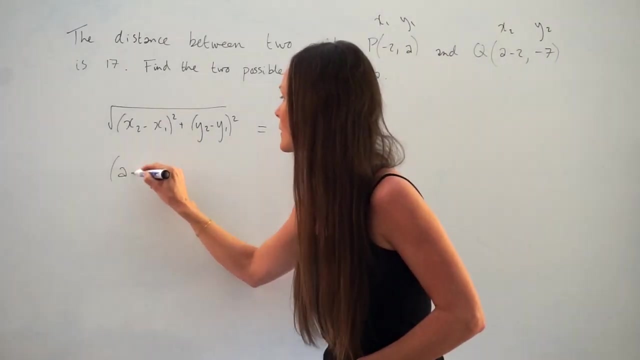 Q is X2, Y2.. And remember, it doesn't matter if you decide to label them the other way around. You'll get exactly the same result. Next, I'm going to substitute my values into the formula. So I need to replace X2 with A minus 2.. And then I'm subtracting every time, remember. 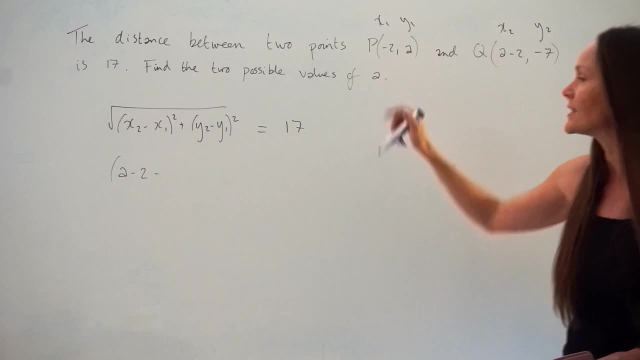 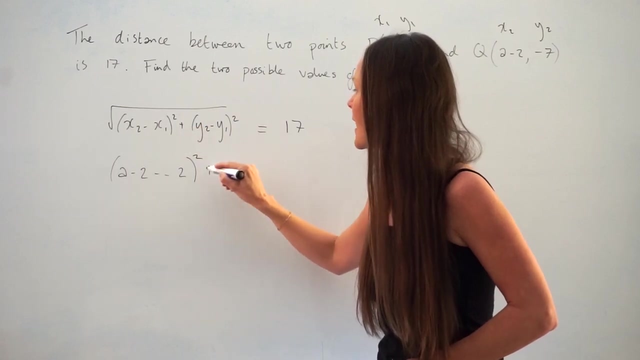 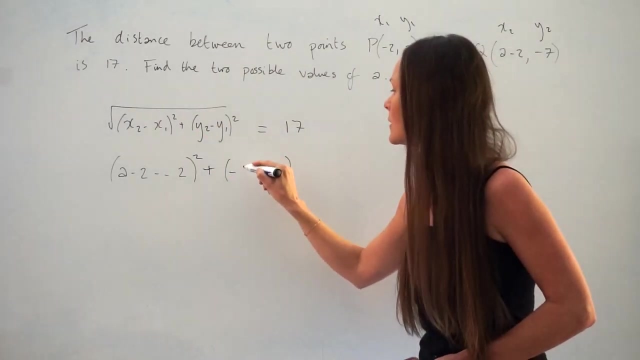 And then I have to substitute in X1,, which is negative 2.. Okay, so watch out, you've got a double negative there. Then we're adding and we're finding the difference between the Y values, starting with Y2, which is negative 7. And you're subtracting Y1,, which is negative. 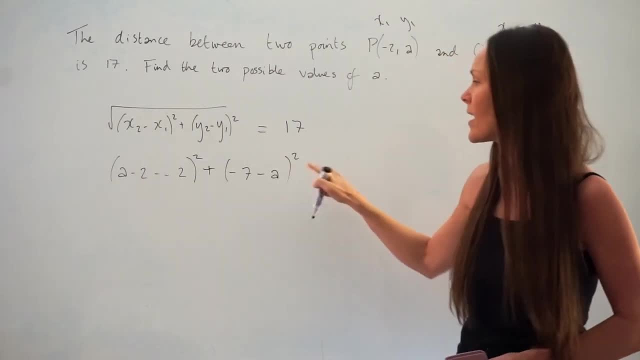 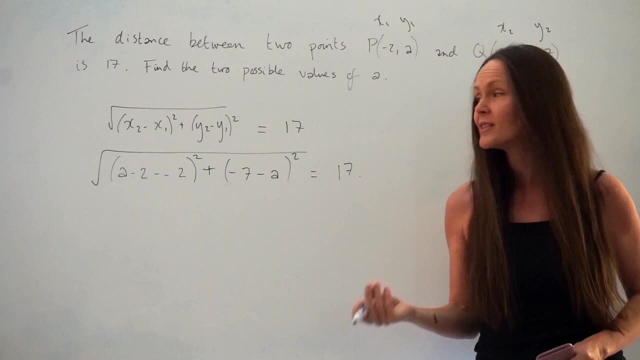 1,, which is F, Not forgetting to square the brackets every time. And that's the square root, and it's equal to 17.. Okay, So I've substituted in my values. Now we have to try and solve this equation. So first I'm going to get rid of this square root symbol. okay. 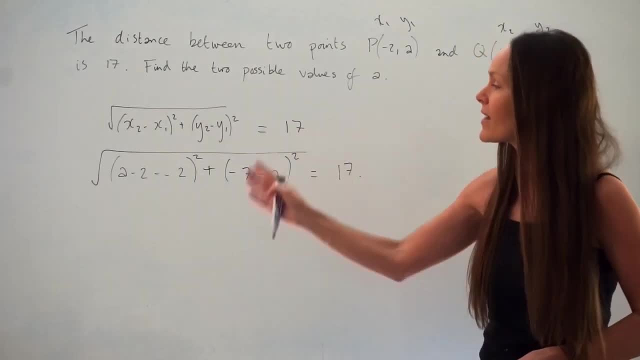 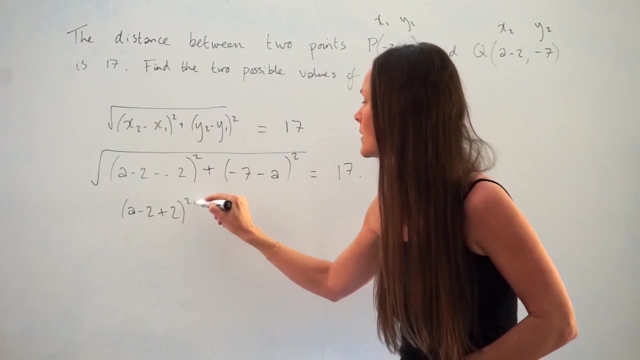 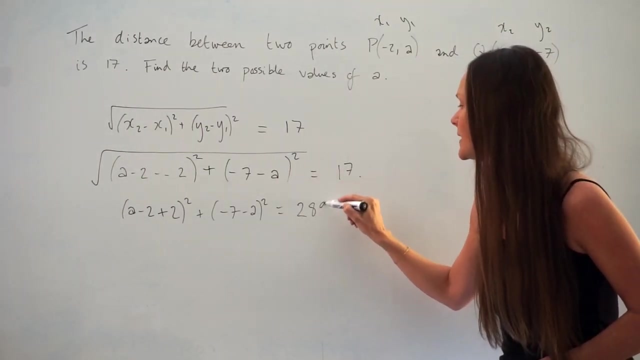 So I'm going to square both sides of the equation. So if I square the left-hand side, I'm just left with A minus 2.. And instead of minus minus 2, I'm going to write plus 2 now, And if I square the right-hand side, I get 289.. Okay, Next we're going to simplify. 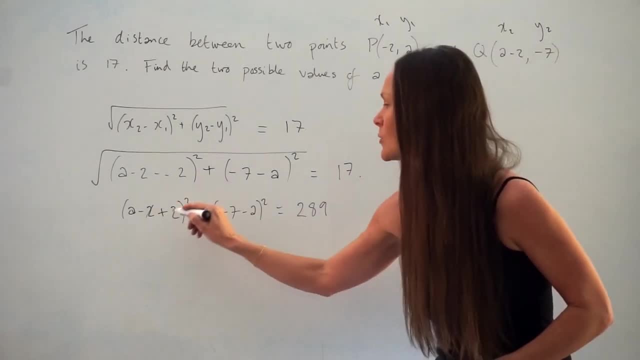 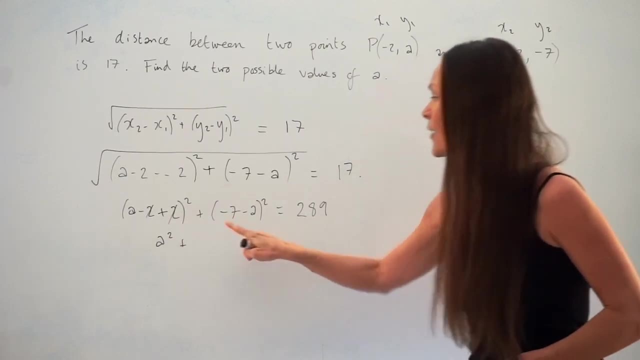 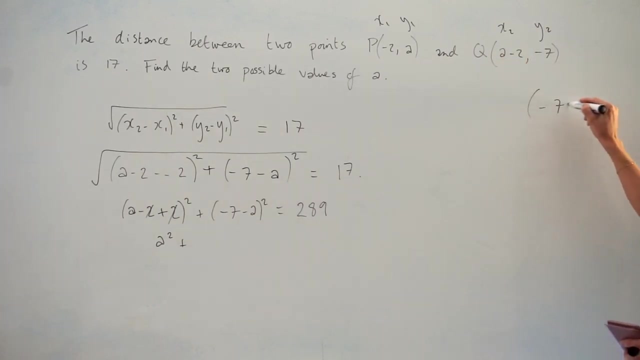 expand the brackets. okay, So I can see minus 2 and 2, they're just going to cancel each other out And if I square A, I'm just going to have A squared If I expand these brackets. remember, squared means multiply that bracket by itself. okay, So it's like saying minus. 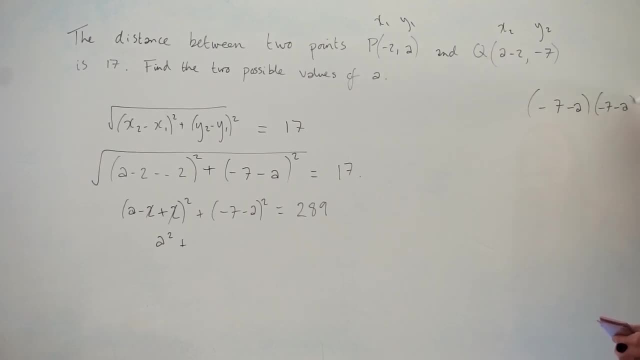 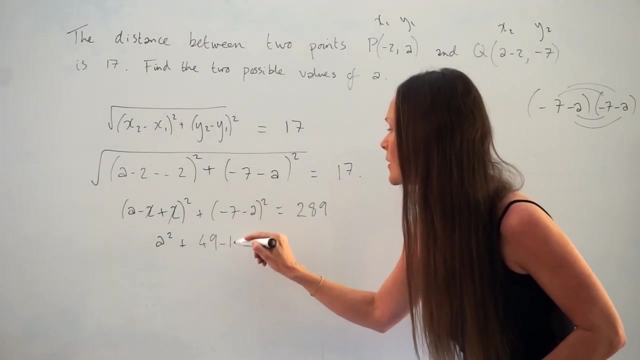 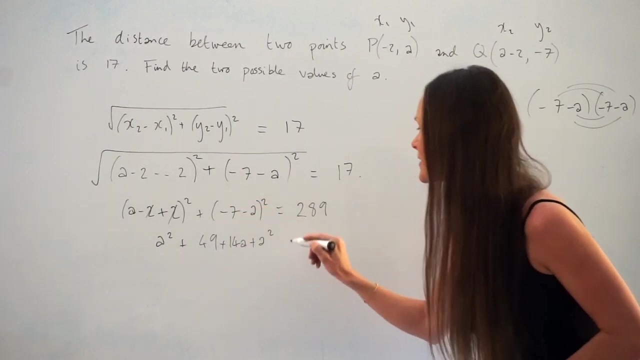 7 minus A multiplied by minus 7 minus A. So I'm going to get rid of this square root symbol. okay. So if you expand those brackets you should get positive 49 minus positive 14A and plus A squared. okay. So that's just expanding those brackets. there Equals 289.. Okay so. 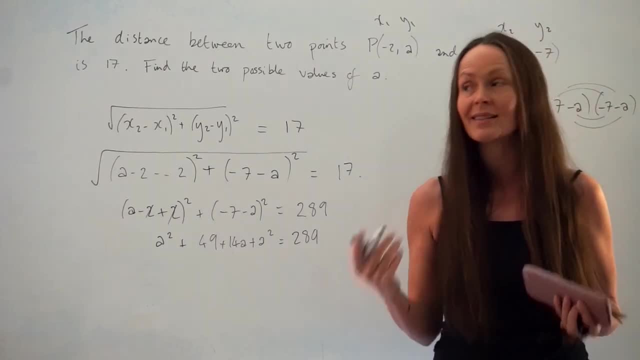 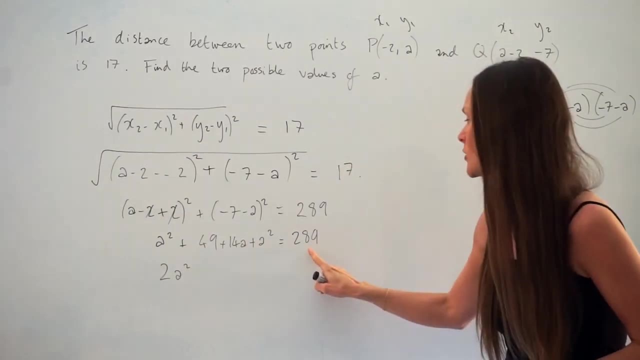 I'm just going to keep simplifying, rearrange the equation so that it's equal to 0,. okay, So I've got A squared plus A squared, which is 2A squared. Then I'm going to move this 289.. 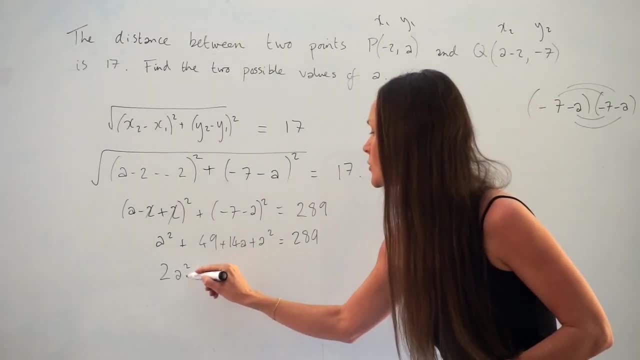 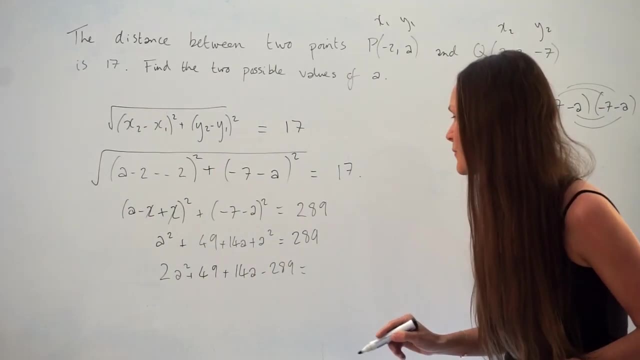 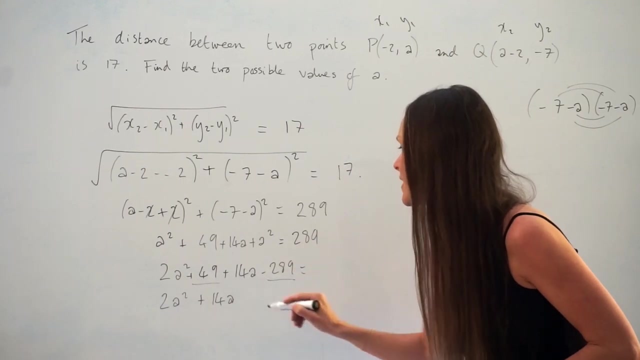 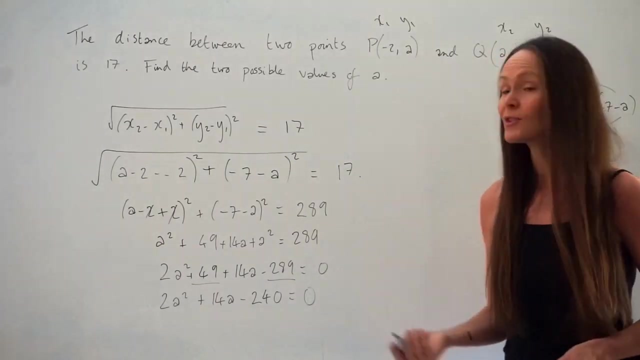 Over to the left-hand side of the equation. So I'm going to subtract the 289.. Then, if I simplify that, I get 2A squared plus 14A, And I'm just simplifying these numbers here to get negative 240.. And remember, this is equal to 0,. okay, Whenever you're solving,